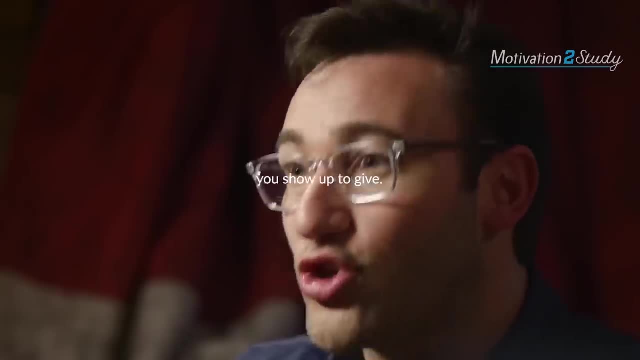 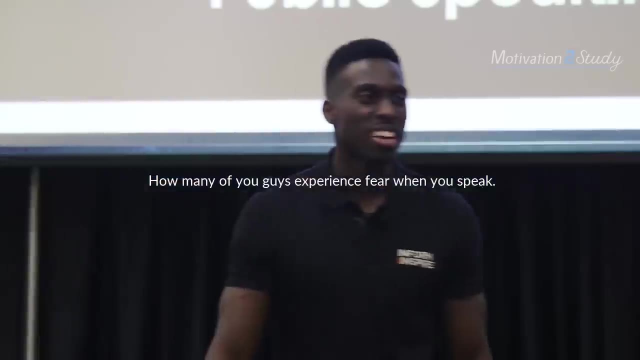 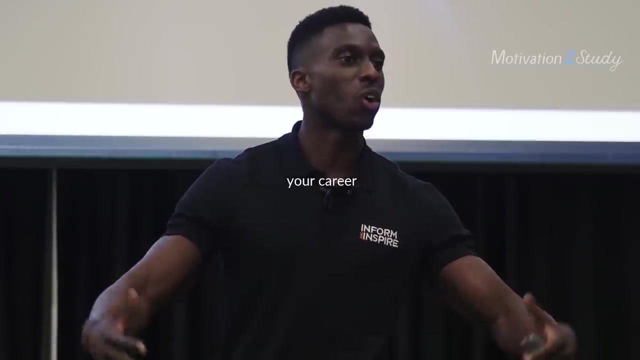 have given them is of value. That's not the reason you show up. You show up to give. How many of you guys experience fear when you speak? How many of you, by show of hands, know that public speaking is fundamental to your industry, your career? By show of hands, How many of you, by show of hands, 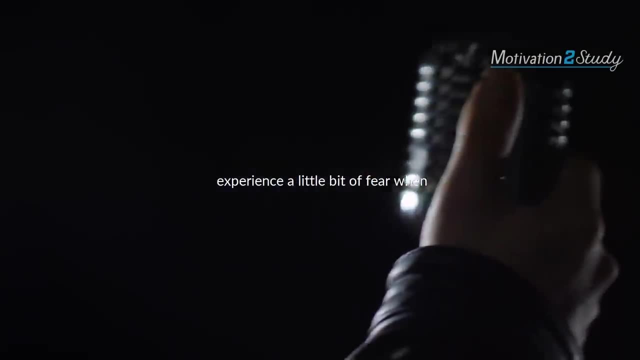 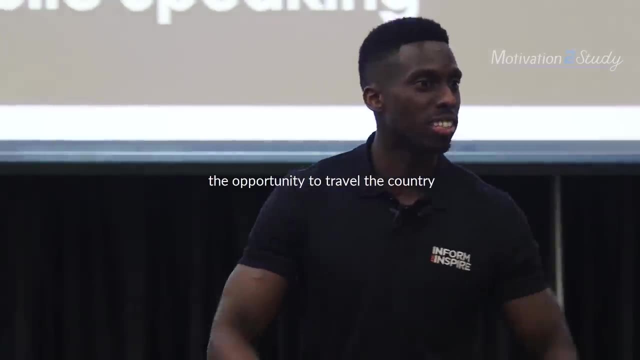 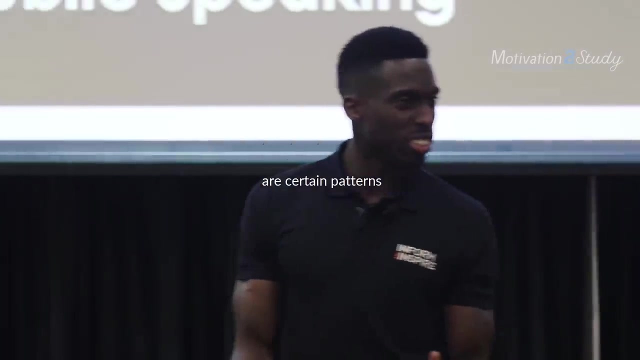 honestly speaking, experience a little bit of fear. when we talk about public speaking, Raise your hand, And over the last three years, I've had the opportunity to travel the country and deliver presentations like this, And what I've picked up on is that there are certain patterns. 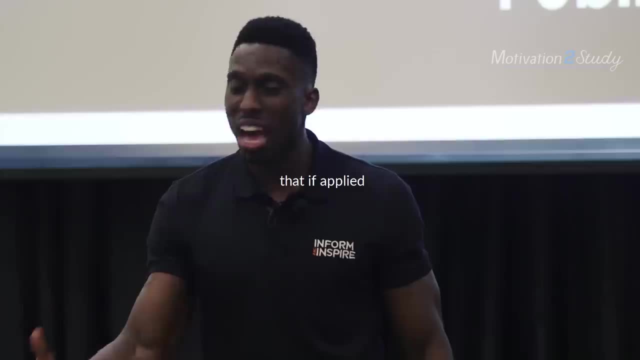 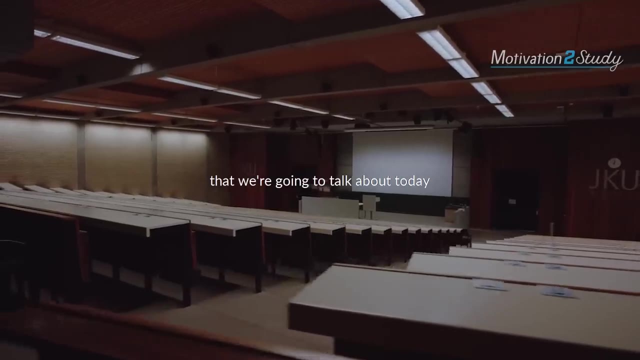 There are certain patterns and certain skill sets that, if applied, can make a public speech amazing. If you follow these principles that we're going to talk about today, I think I don't care what industry you're part of, I don't care what work you're in. 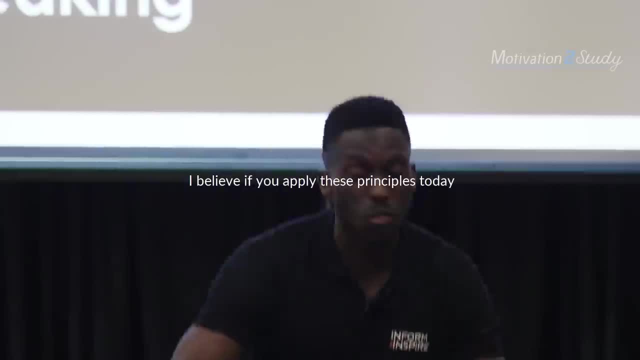 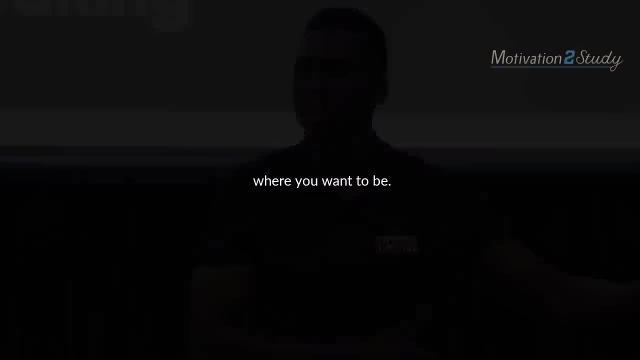 I don't care what year you are, I don't care how old you are. I believe if you apply these principles today, you can literally transform where you are and take the journey to where you want. to be Straightforward, I believe there's three principles, three A's of public speaking. 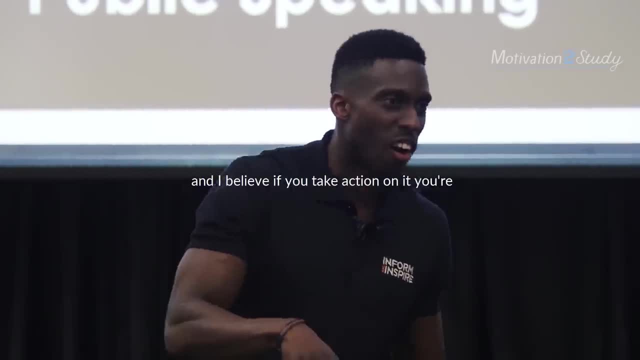 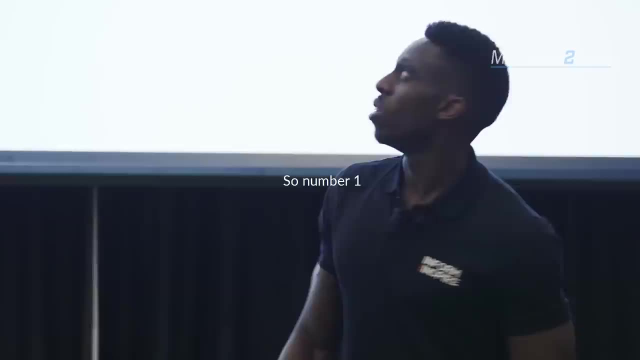 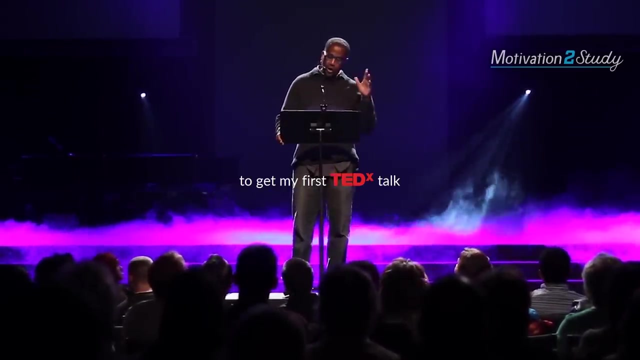 that I want to leave you with today And I believe, if you take action on it, you're going to be like: oh my God, I'm glad I came. So number one: authenticity engages. November 2017, I was afforded the opportunity to give my first TedX talk and, man, can I tell you, 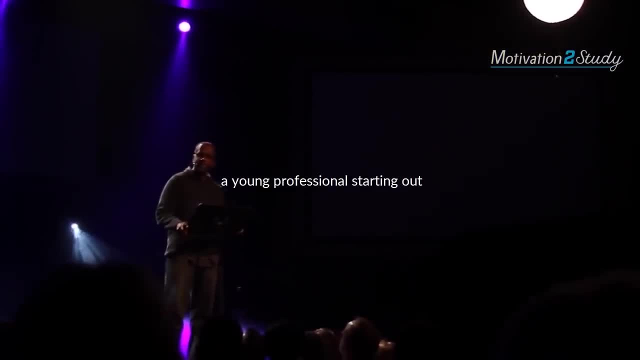 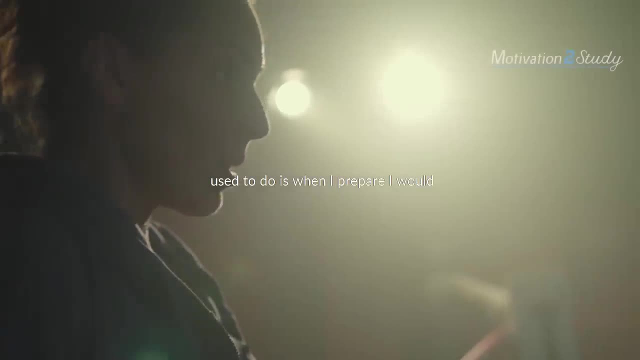 I was excited. You've got to imagine a young professional starting out, ready, 26 years old, And I want to make this very clear. So I'm thinking to myself, And what I used to do is, when I prepare, I would give a talk at least a hundred times. 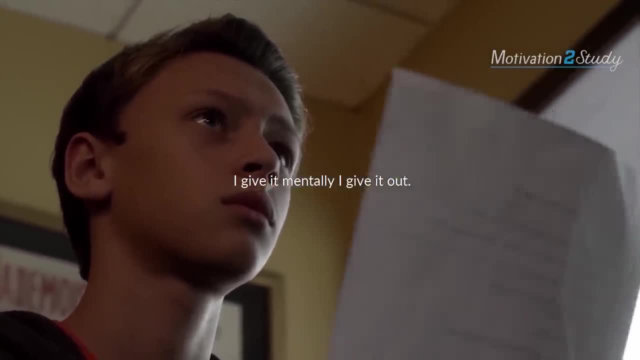 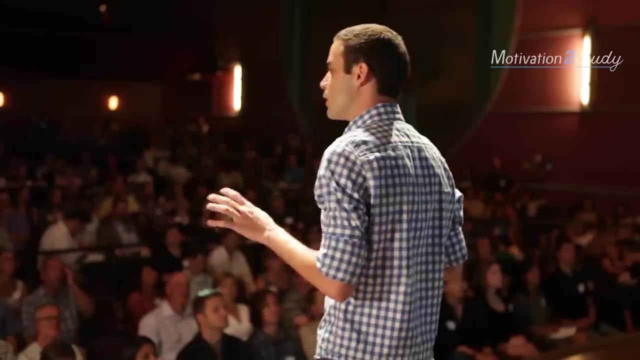 Before I give it, write that down, I give it mentally, I give it out. I talk to people conversationally In the shower I'm like, okay, this is okay, alright, I'm going to do this right. And I think to myself: PowerPoint or no PowerPoint. 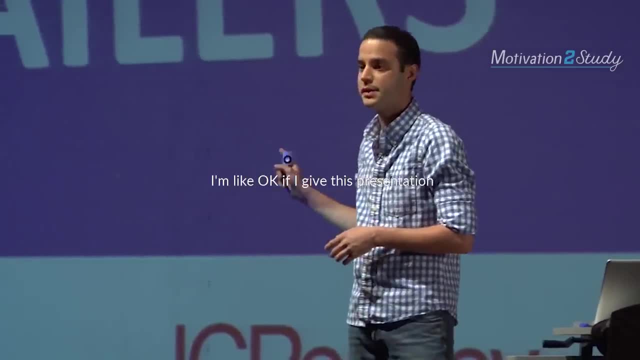 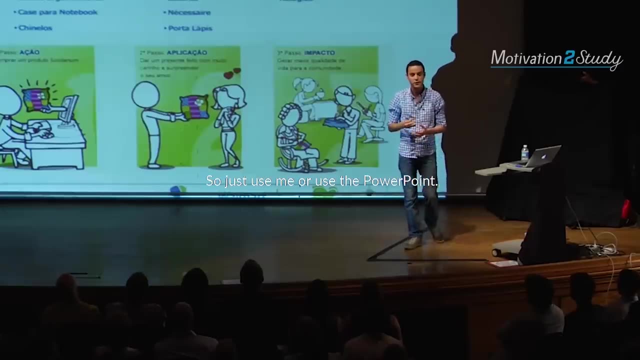 That's all I'm thinking. I'm like, okay, If I give this presentation, Should I use the PowerPoint behind me, Or should I just use me, Or should I use the PowerPoint? So I'm researching and I'm watching. I've watched more TED Talks than you could possibly imagine. 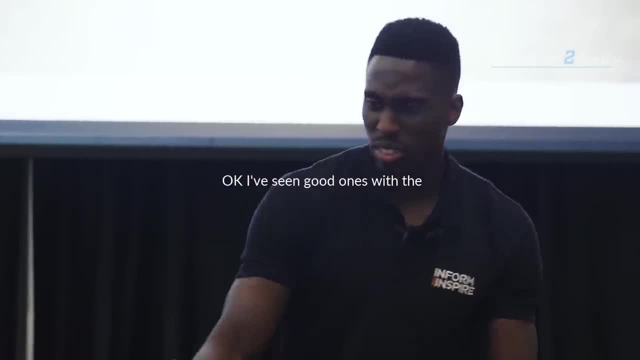 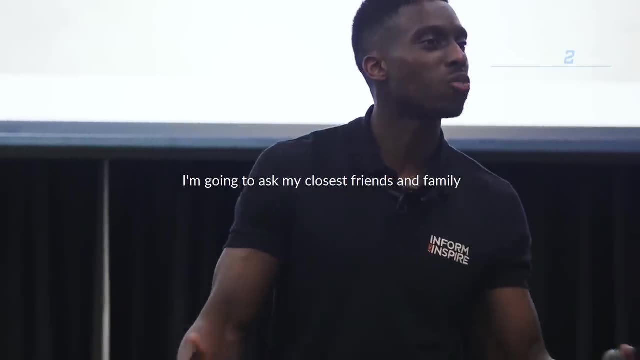 And I'm like, okay, they do this, they do that. Okay, I've seen good ones with the PowerPoint, I've seen good ones without. And what I notice is- I said you know what I'm going to ask my closest friends and family. 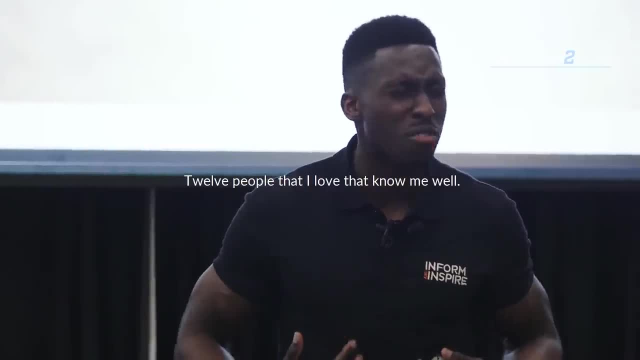 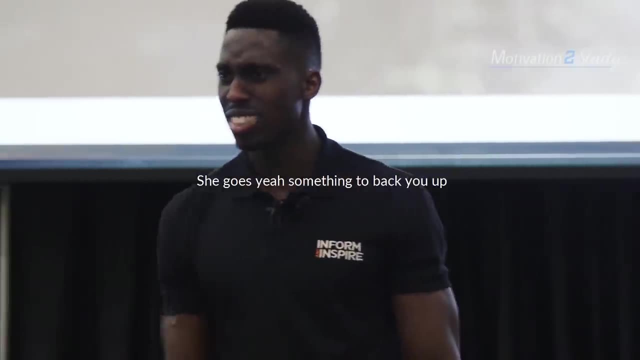 I'm going to take a poll. Twelve people that I love That know me well. I said: sister, Should I use a PowerPoint? She goes: yeah, Something to back you up, Use a PowerPoint. I go: mom, Should I use a PowerPoint? She says no PowerPoint. 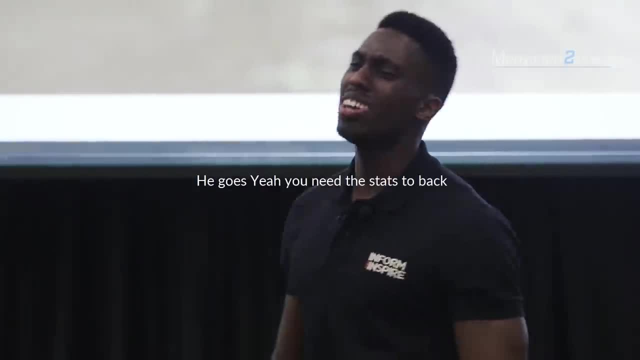 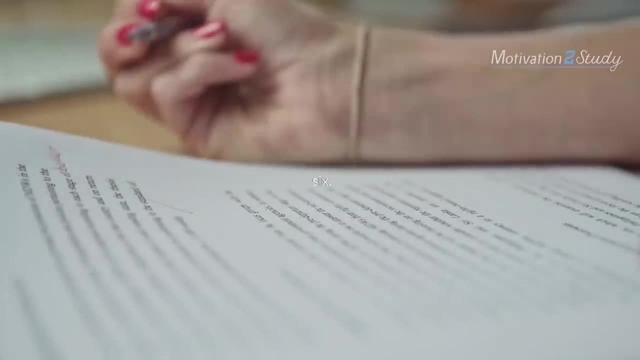 Use you. I say, bro, Should I use a PowerPoint? He goes, yeah, You need the stats to back up what you've done. I said, cool, I go through the entire list. Six, six. I put the list down and I go. What was I thinking? 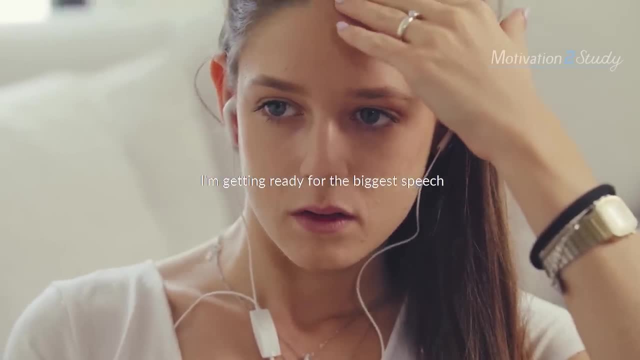 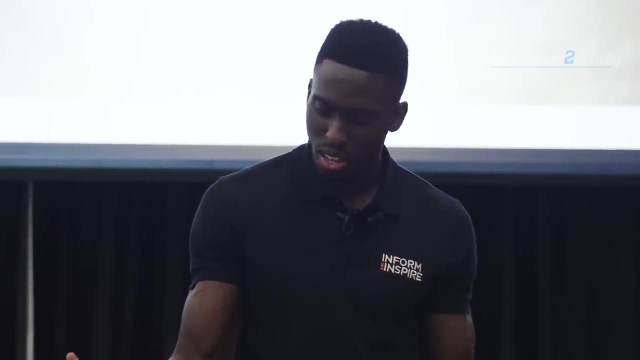 With an even number. I'm getting ready for the biggest speech of my professional life. Right And professionals, People that I love- Are telling me: no, PowerPoint, PowerPoint, And it's 6-6. And I'm like: how am I going to break this tie? And I'm like: wait. 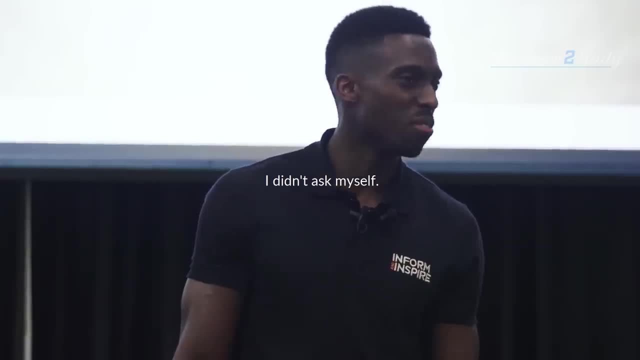 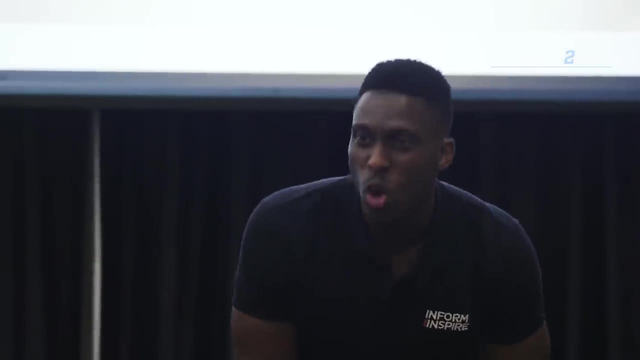 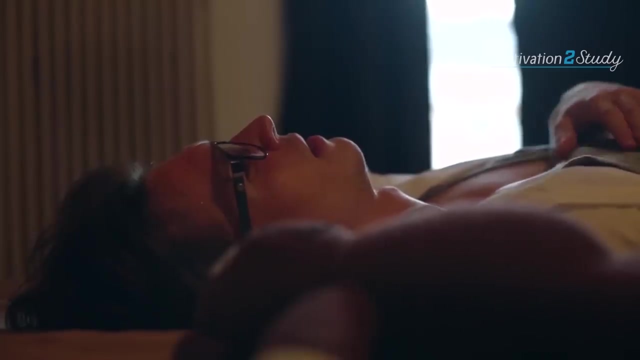 I didn't ask one person. I didn't ask myself. I did not ask myself What I would be most comfortable with To present When we talk about public speaking And why I say authenticity engages. Listen to me here. Listen to me here. You have to know yourself Before you go and seek advice. 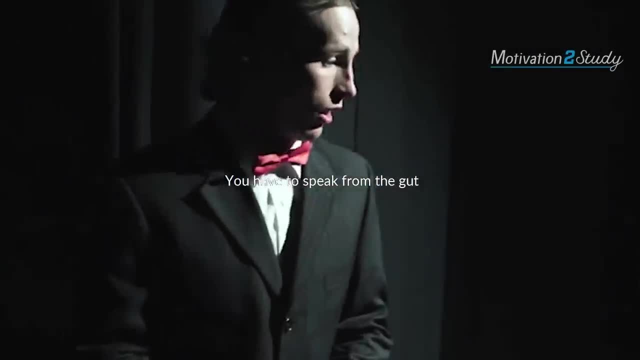 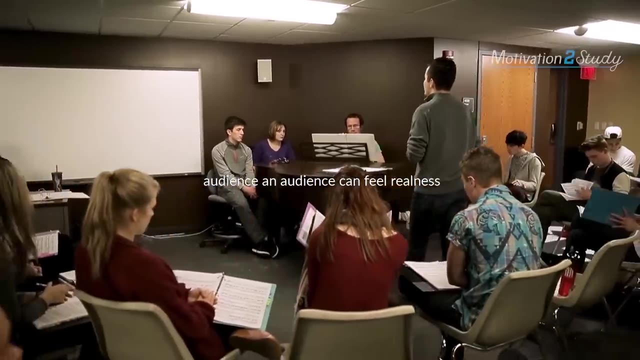 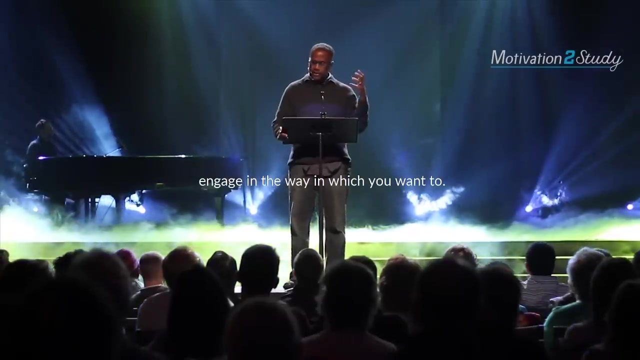 You have to speak from the gut Before you go and ask, Because when you're talking to an audience, An audience can feel realness And you have to be yourself. If you can't be yourself, You will never engage in the way in which you want to. That I have to listen to me first. 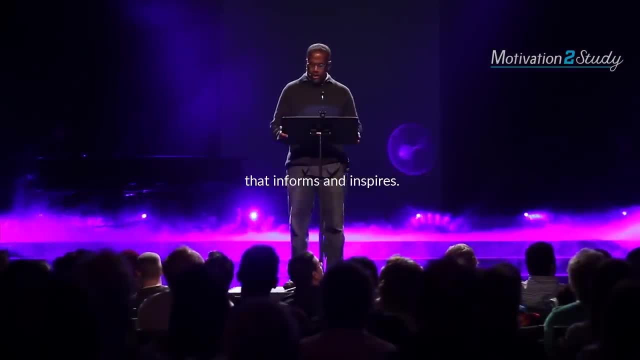 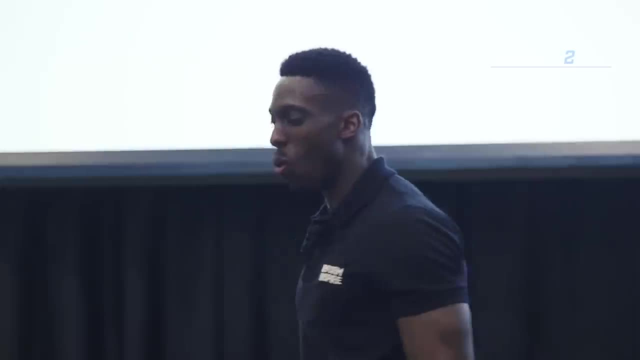 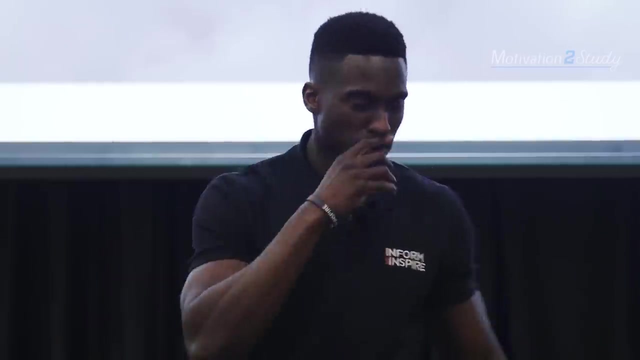 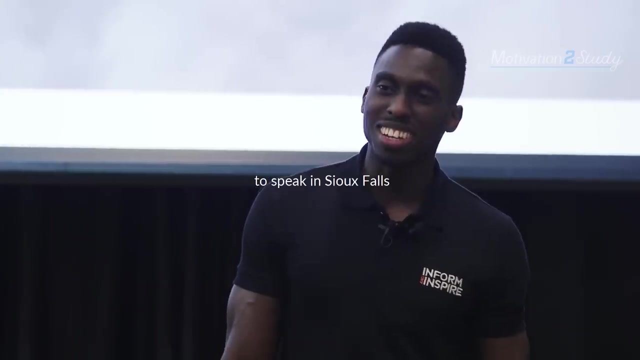 In order to really deliver a message, informs and inspires. Number two: awareness Awareness connects the speaker to the audience, and this is what I mean, And so one of the speaking events comes, comes about and I get the opportunity to to speak in Sioux Falls, South Dakota, and 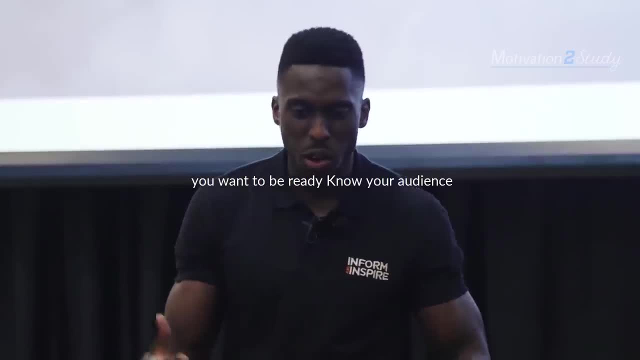 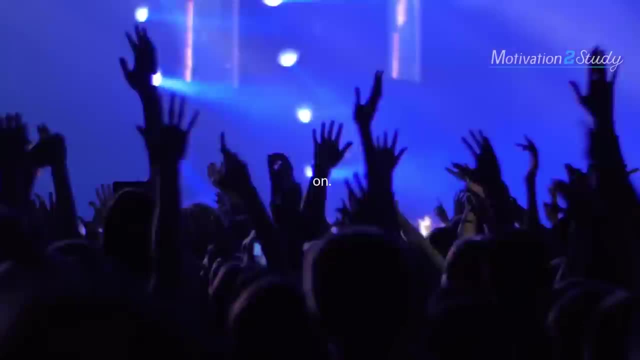 before the event. you know you want to be early, you want to be ready, know your audience, know your crowd. I hear like all this partying type thing going on. I'm like what's going on and I go down and they have, they have an open bar and they. 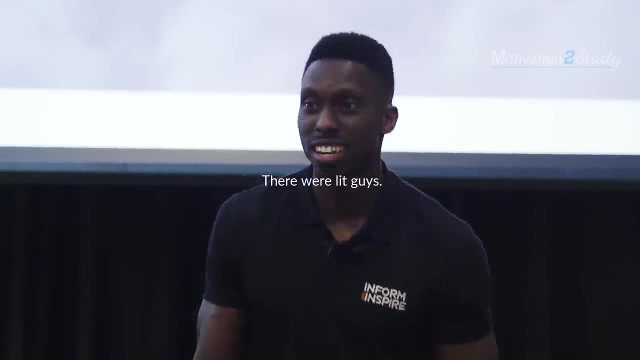 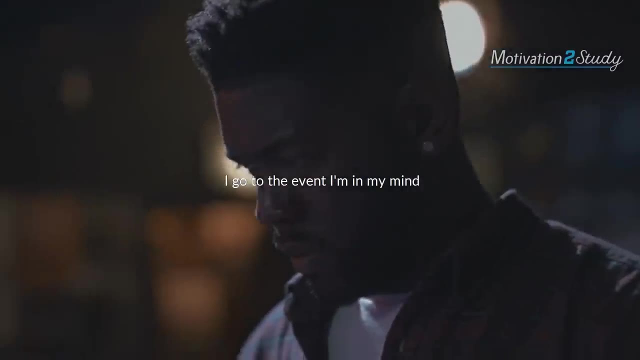 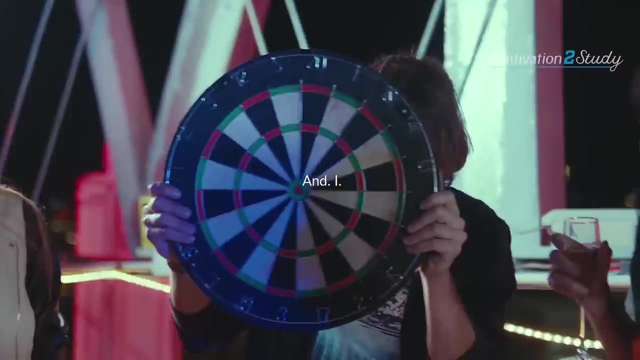 had the open bar for hours. They were lit guys, They were lit right, And so, listen, I go to the event. I'm in my mind, I'm thinking it's going to be a, a, a, a professional, motivational. this is what you need to do and I walk into a party. 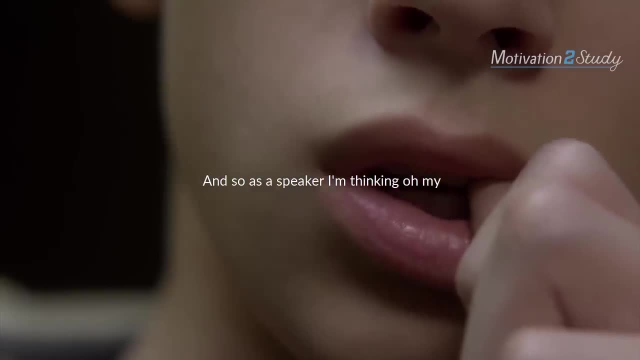 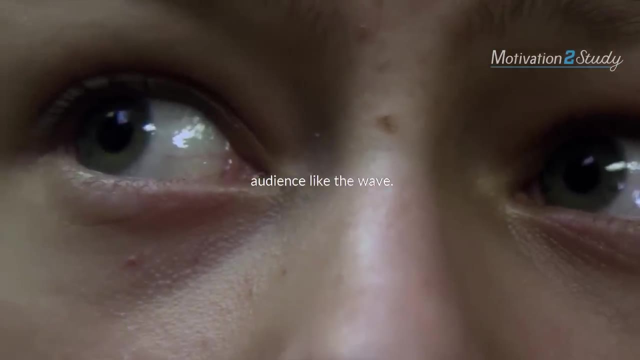 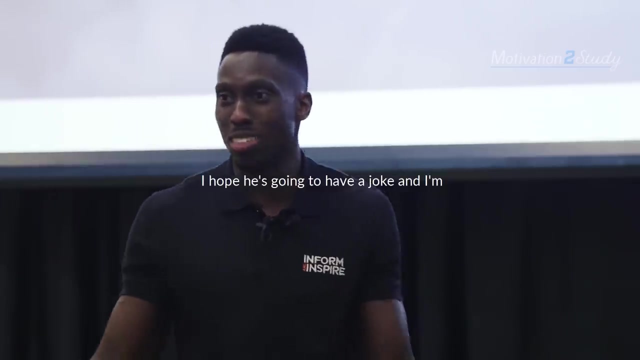 and so, as a speaker, I'm thinking, oh, my goodness, like I was prepared to do one thing, I flew all the way here and there's literally a party in the audience like the, the wave, the energy is like: hey, I hope this guy's cool, I hope he's gonna, you know, have a joke, and I'm like that's not the. 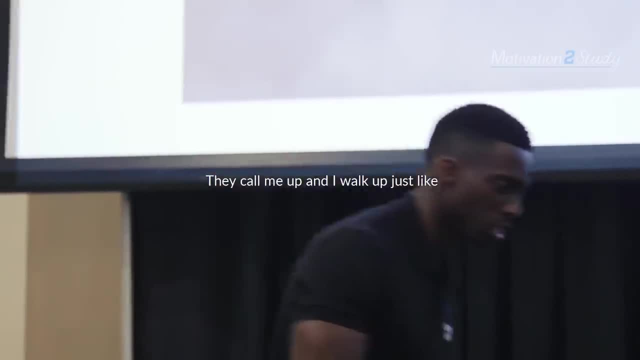 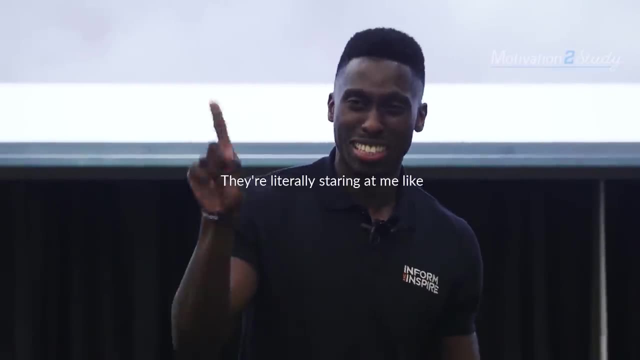 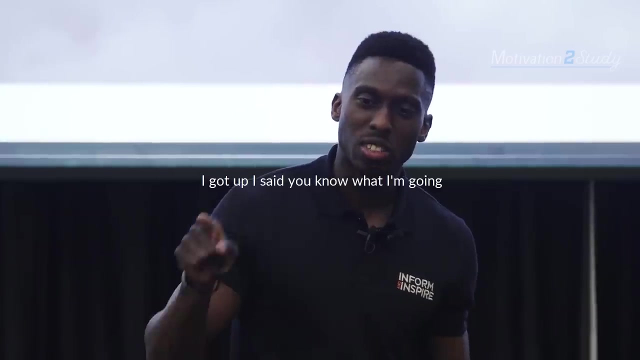 content that I delivered. so I get up, they call me up and I walk up just like this, and they're as quiet as you guys are. they're literally staring at me like what's this guy about, right? and at that moment I decided, right before I got up, I said: you know what I'm gonna. 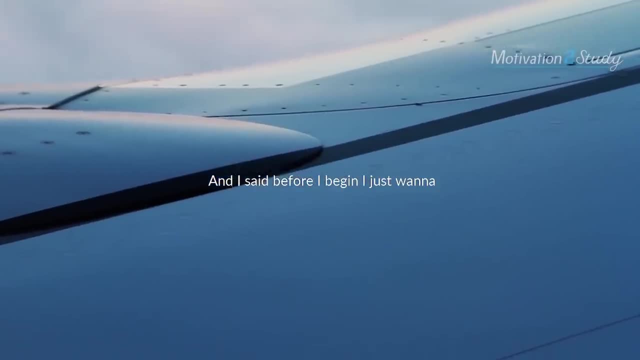 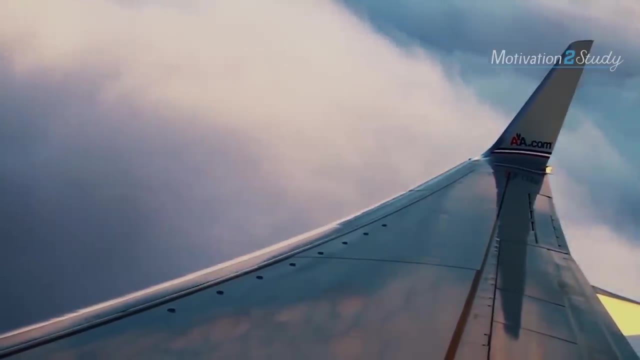 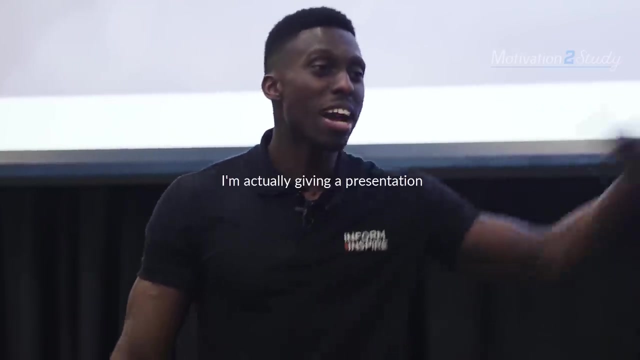 tell a story. and I said before I begin, I just want to let you guys know I'm. I'm coming from Sacramento and I hopped on the plane and I met an individual and we're chatting it up and he thought I was going to give a presentation in Colorado and I told him: no, I'm actually giving. 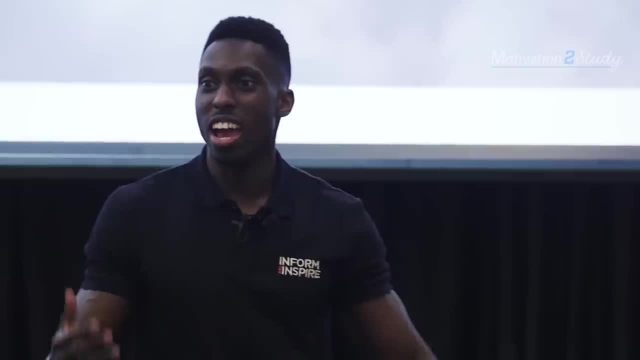 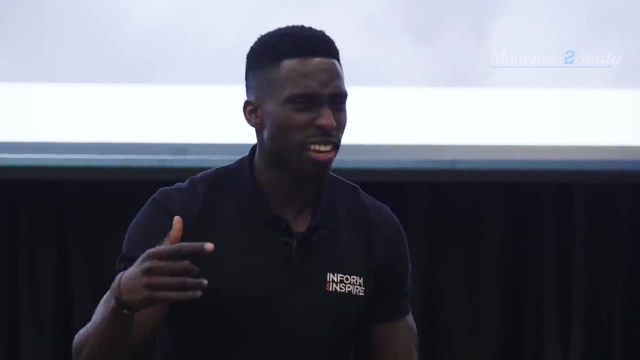 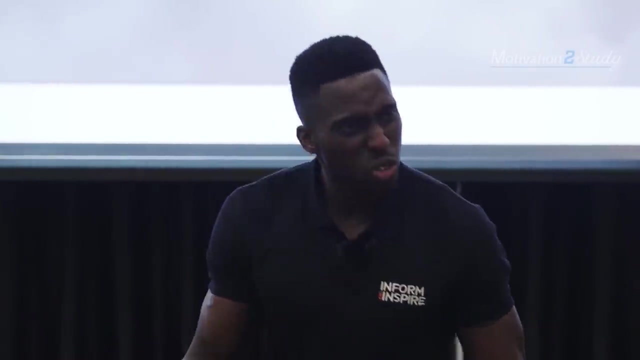 a presentation in Sioux Falls, and the look on his face was blank and I and he said, excuse me, where? and I said Sioux Falls. then he said these three words and I'll never forget it. he said: are you sure? and I said that. and there was a man sitting right where you're sitting. 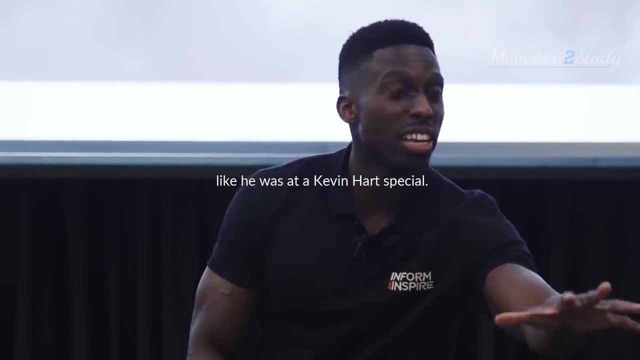 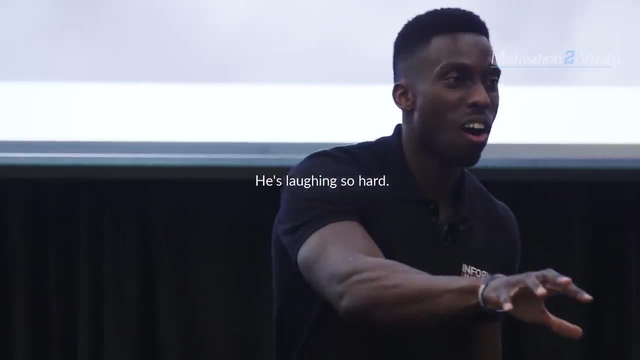 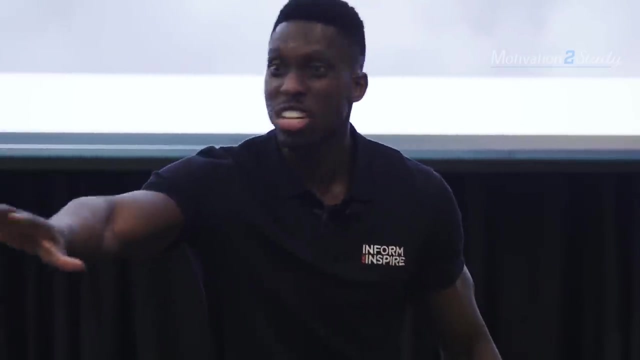 and he literally laughed like he was at a Kevin Hart special. he lost- I'm talking chair went back. he's laughing so hard- it's about a crowd of 200- that everybody you guys ever caught this. when somebody laughs so hard that you have to laugh, the whole crowd literally just starts busting laughing. and I start laughing from the stage. 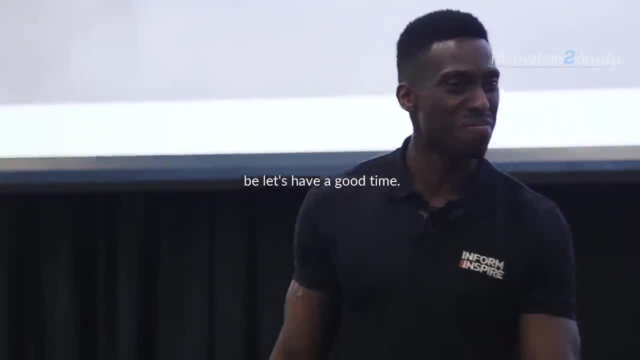 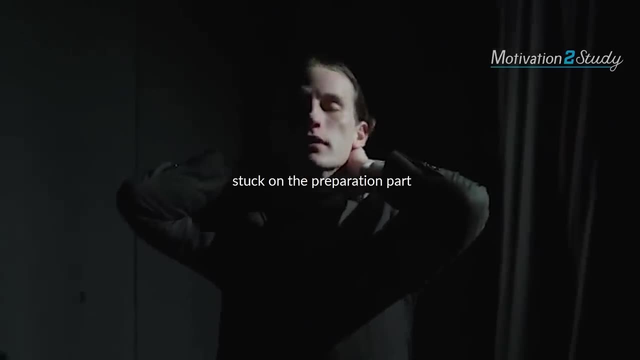 I'm like, man, if this is how it's gonna be, let's have a good time. and at that moment I'm like: oh, that moment I realized something, because the old me would have been so stuck on the preparation part that I would have never had the audacity I would have. 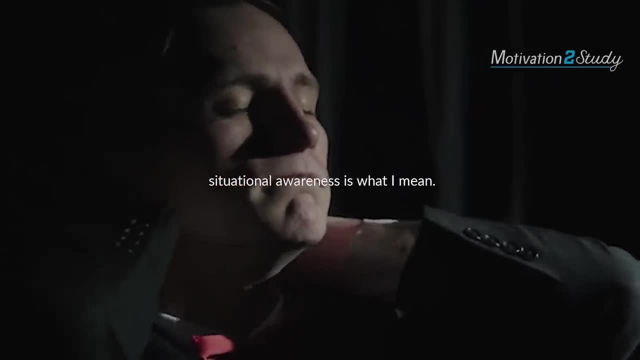 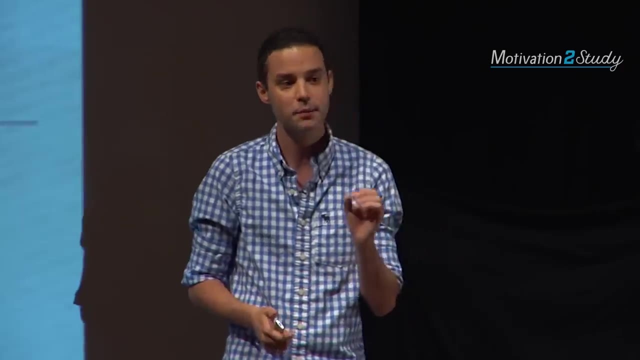 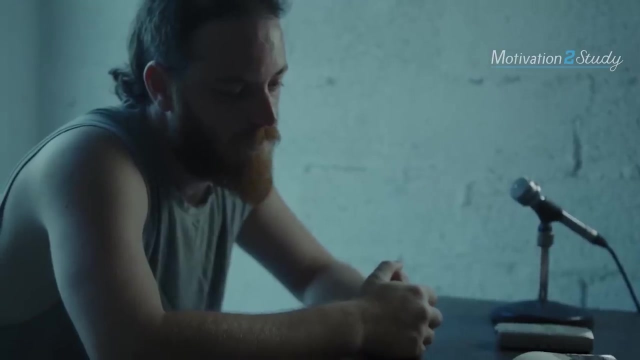 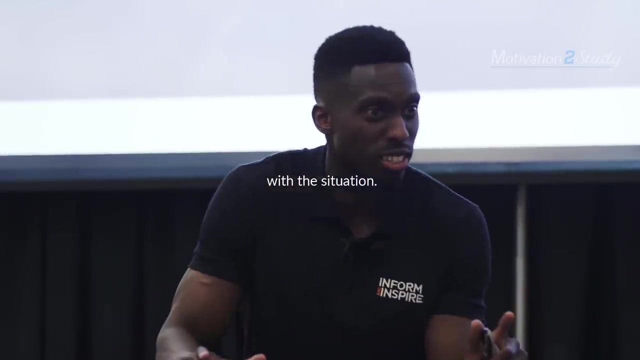 never had the awareness. situational awareness is what I mean when you speak or present. sometimes things will not go as planned and there's no way to plan for it and what you have to do is be fluid and malleable and ready to rock with the situation. and if you have situational awareness, what often can? 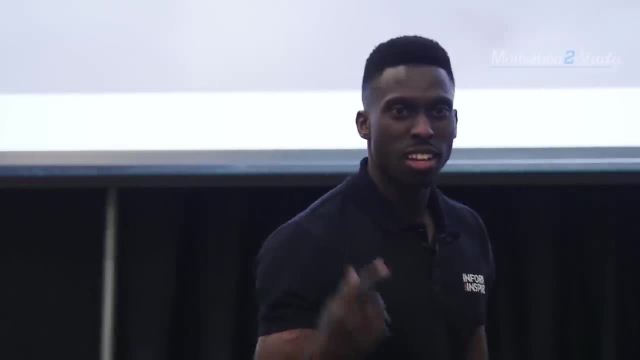 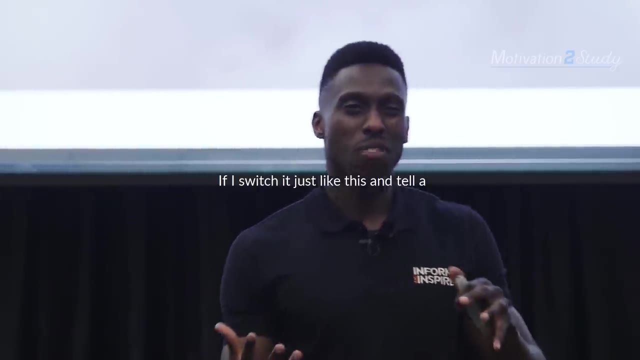 happen is you can play on what is happening. I said huh, open bar, alcohol, social event. I'm coming with motivation. if I switch it just like this and tell a joke and let them know I'm not all serious up here, the audience will be on my side. 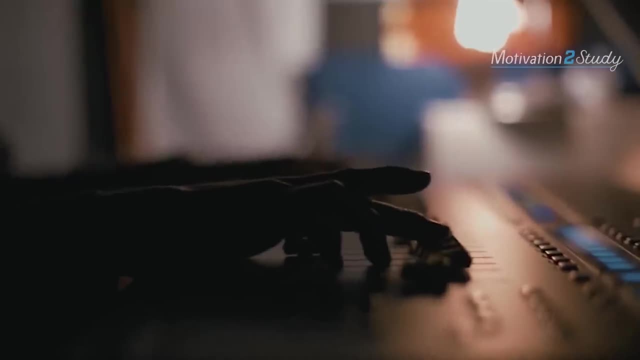 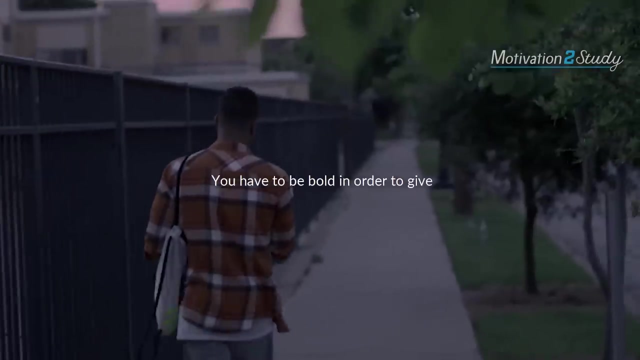 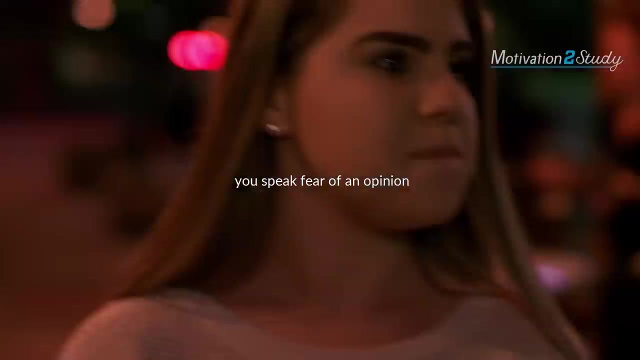 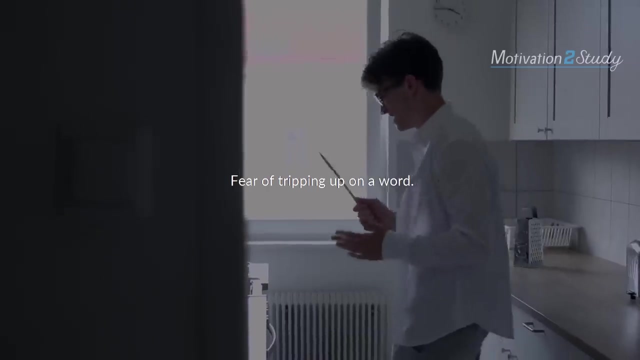 number three: audacity. audacity informs and inspires. you have to be bold in order to give a speech that's going to last. how many of you guys experience fear when you speak? fear of an opinion of other, fear of being criticized, fear of not being good enough, fear of tripping up on a word, fear of what you? 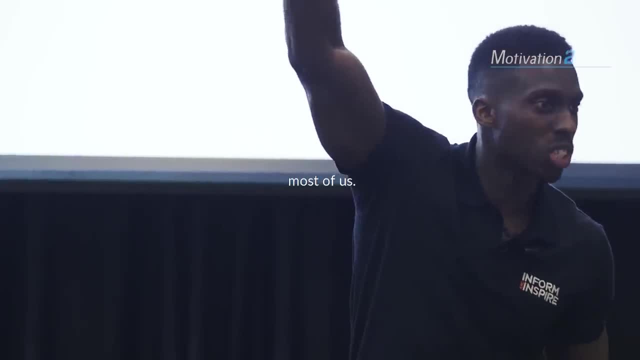 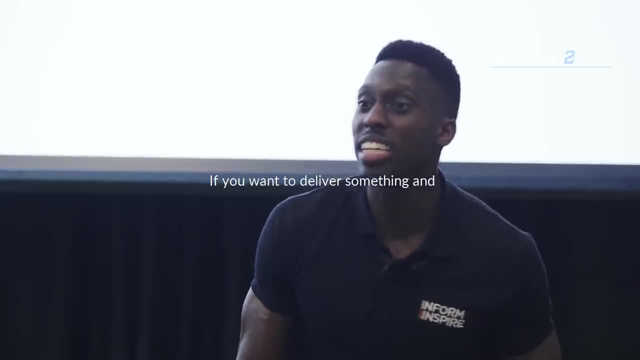 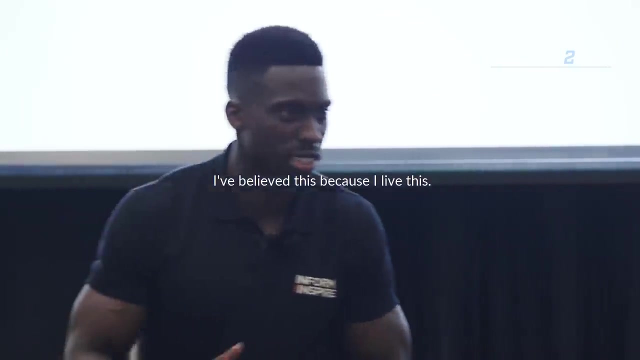 look like. we know that fear drives most of us, and I'm here to tell you that audacity is what you need. boldness is what you need if you want to deliver something and absolutely be transformative. I'm passionate about this. I believe this because I live this. I'm telling you, you. 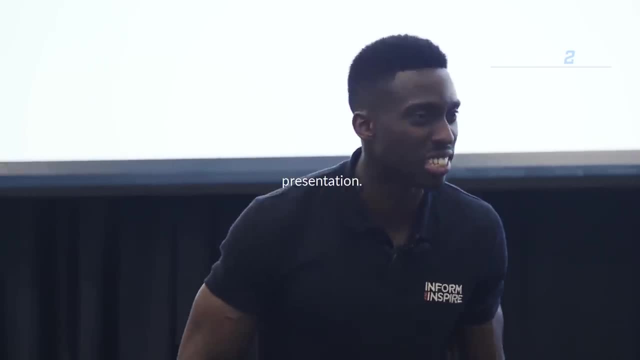 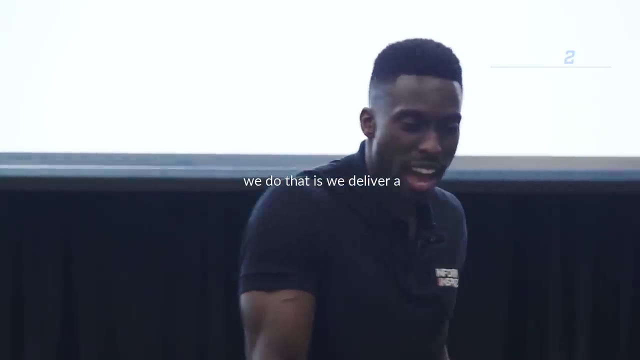 have to be bold. you can't half step into your presentation. you have to be bold. you cannot half step into your presentation, and one of the ways in which we do that is we deliver a story. story includes power, words and words, and- and I promise, because I say this word forced- it's automatically reflected into